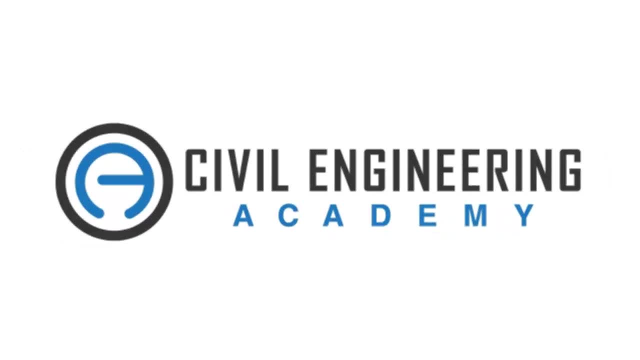 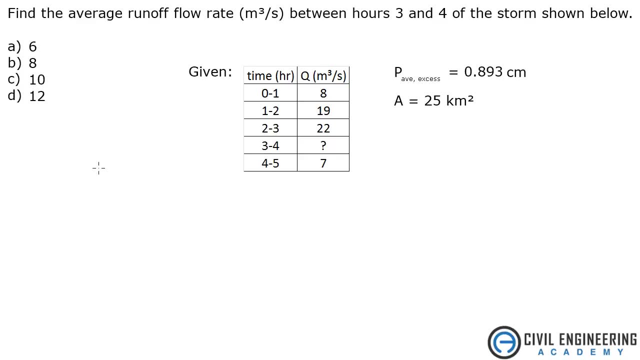 Civil Engineering Academy. Hey, what's up everybody? Welcome to Civil Engineering Academy. Today we're solving a problem from hydrology. The problem states: find the average runoff flow rate in meters cubed per second between hours three and four of the storm shown below. 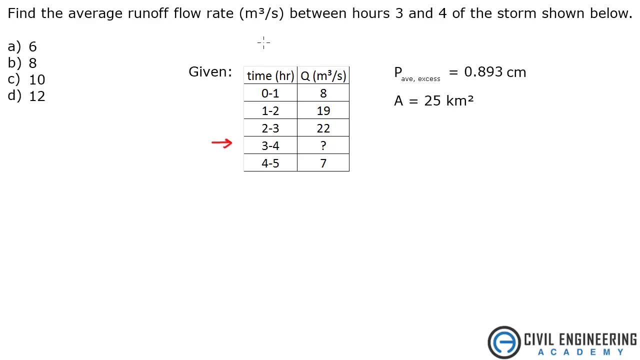 So we're asked to find hours three to four, which is found right here. This is called a hydrograph And if you're using the Civil whoops Civil Engineering Reference Manual, chapter 20 goes over hydrographs. Basically you could plot this: a, Q versus T. 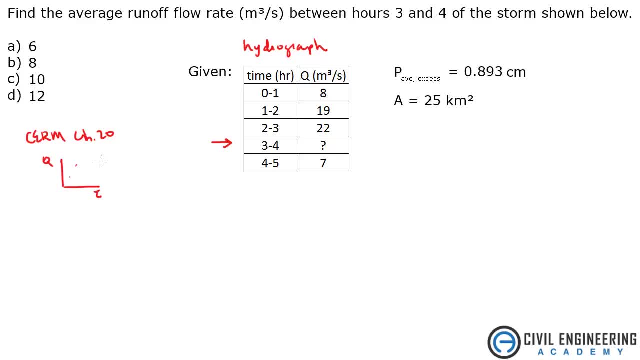 and on hour one you'd have eight, 19,. hour two, 22,. hour three, we don't know. hour four is seven and you develop some sort of curve like this and we're trying to find the value right there at this time: three to four hours. 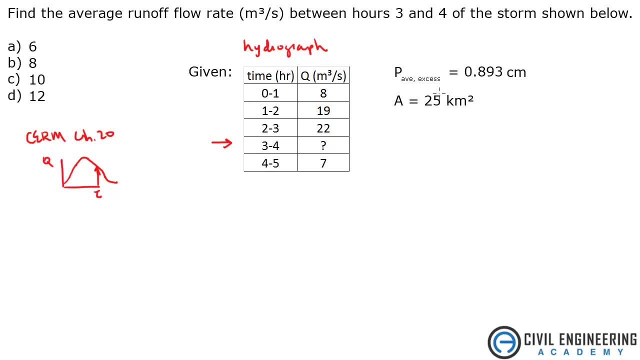 So how are we going to do this? We're also given the excess precipitation and the area. First thing we're going to do is we're going to know. we know that volume equals time times, flow rate, And so in this case we have all these different flow rates. 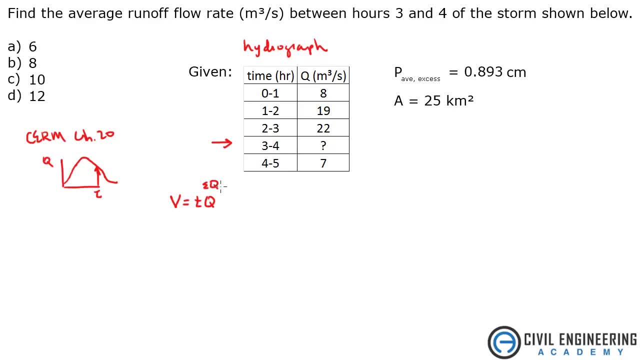 so we're going to sum up the flow rates and we need to solve for this hour. So I'm going to call this Q one, two, three, four, five and we're going to rewrite this basically to this volume equals time times: Q one plus Q two plus Q three. 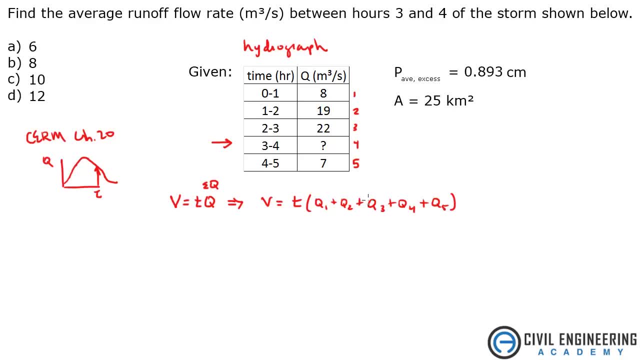 plus Q four, plus Q five, And then I'm going to rewrite it in terms of Q four, because that's the one that we want. So Q four is going to equal our total volume divided by time, minus Q one, minus Q two, minus Q three. 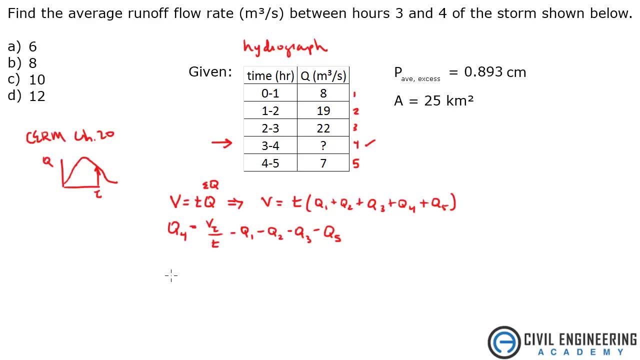 minus Q five. So all right, we got that set up. The next thing we need to do is use equation 20.21 in the civil engineering reference manual. that states that our total volume. Total volume is equal to the area times the excess precipitation.